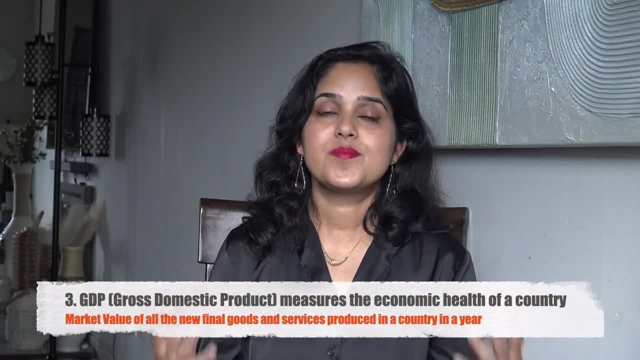 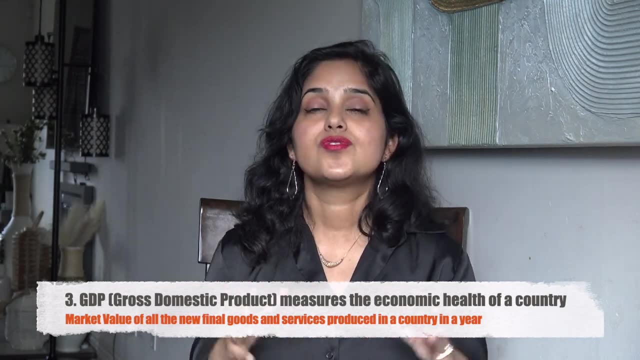 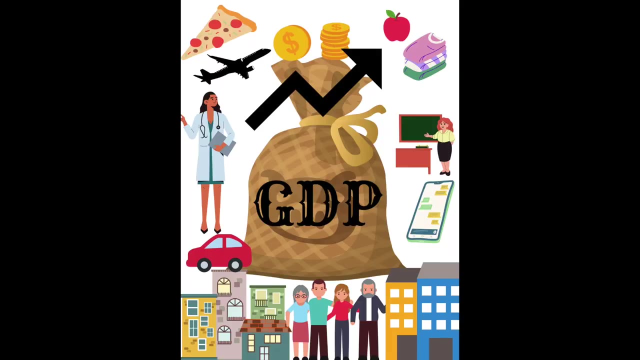 It tells how much money the people in the economy and the businesses have made in one year. So GDP is a measure of the economic output of a country and is used to track the overall health of the economy. It represents the total value of goods and services produced within a country's. 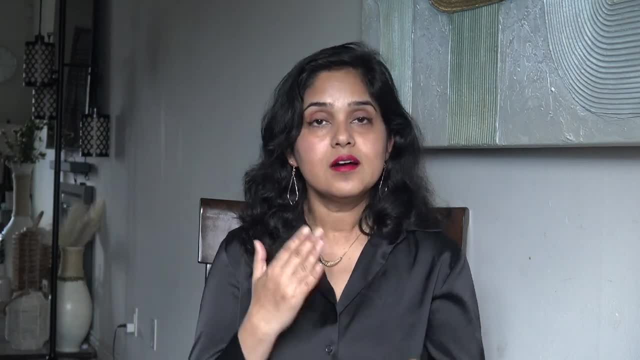 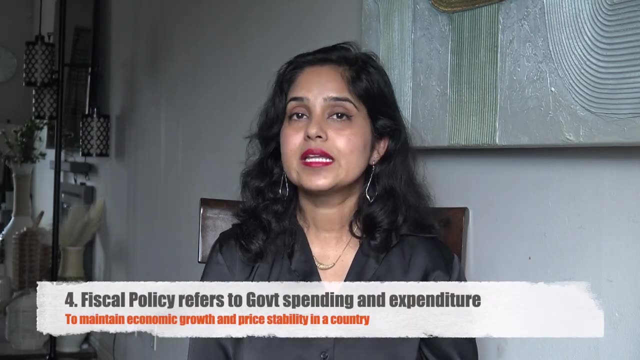 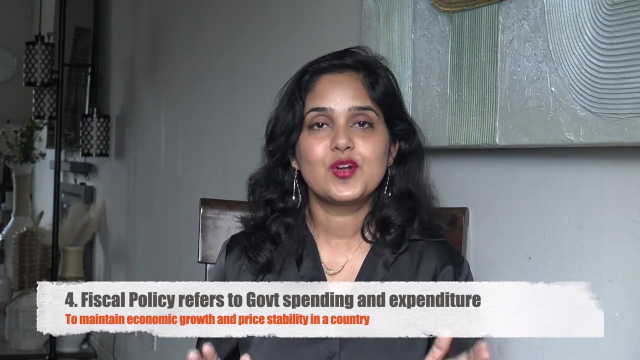 border in a given period of time, typically a year. The next important concept that you should know about is called fiscal policy. The government can help the economy by spending money when things are bad and not spending as much when things are good. So the fiscal policy refers to the taxation. 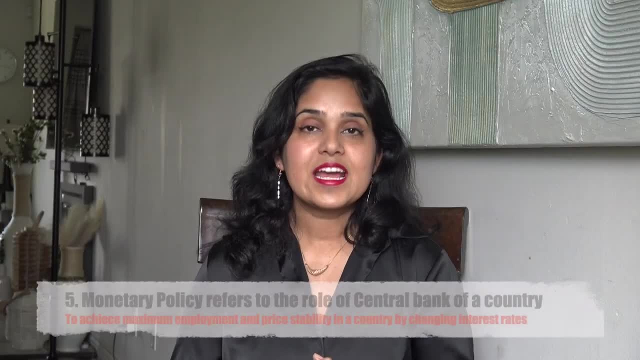 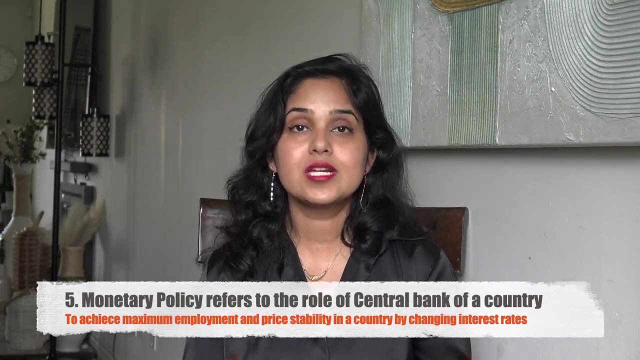 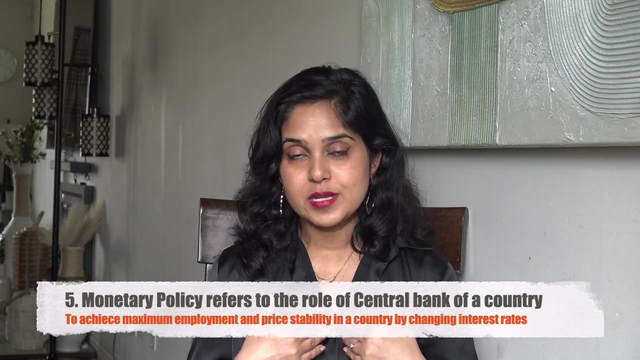 and spending behavior of the government. The next important concept is monetary policy, So the government can also help the economy by changing how much interest people have to pay when they borrow money. This can make it easier or harder for people like you and me to buy things. 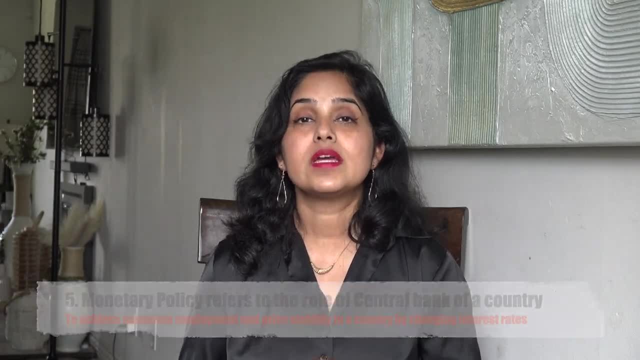 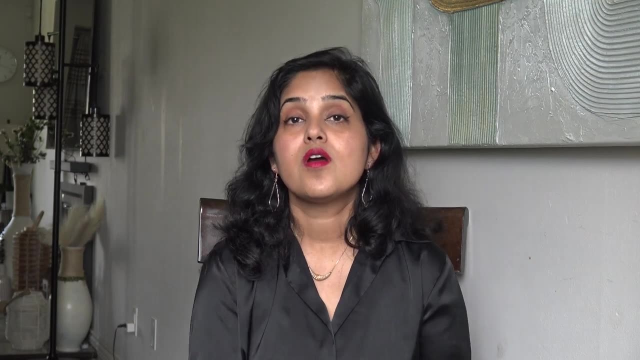 So, in other words, monetary policy is the use of interest rates and other tools by the central bank to manage the money supply and influence economic activity. For example, we can adjust the minimum interest rate in a country by using the money supply policy or the interest rate review. 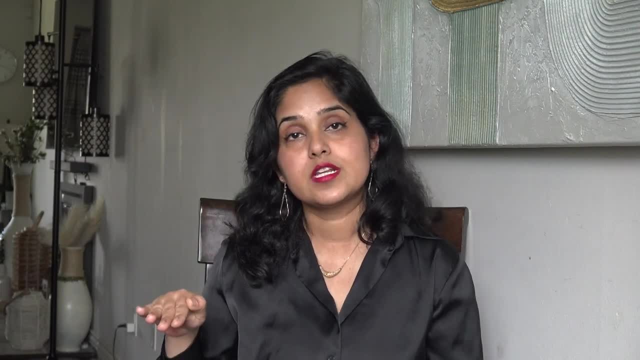 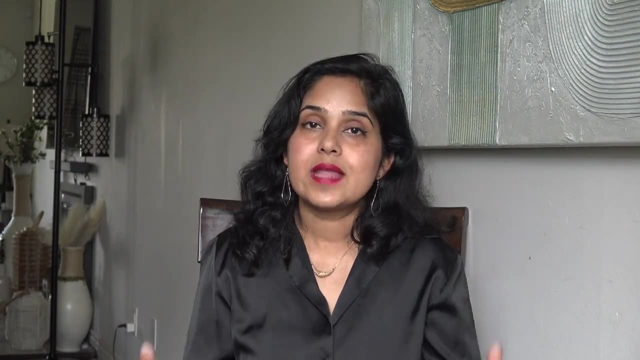 scheme, For example. we can solve the interest rate crisis by accessing and selling books, For example. example, a central bank may lower interest rate to encourage borrowing and stimulate economic growth, or can raise interest rate to cool down inflation. The next important concept that everyone should: 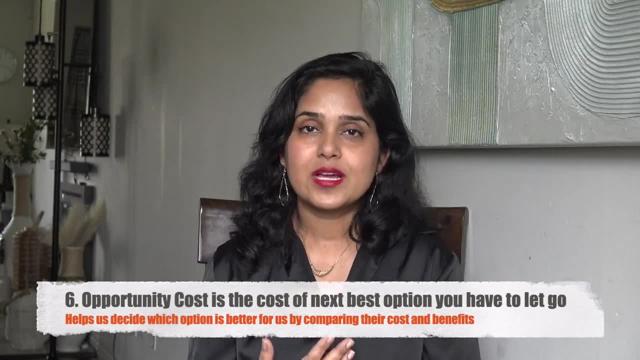 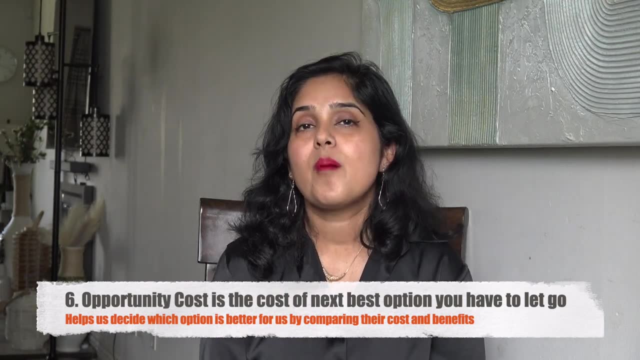 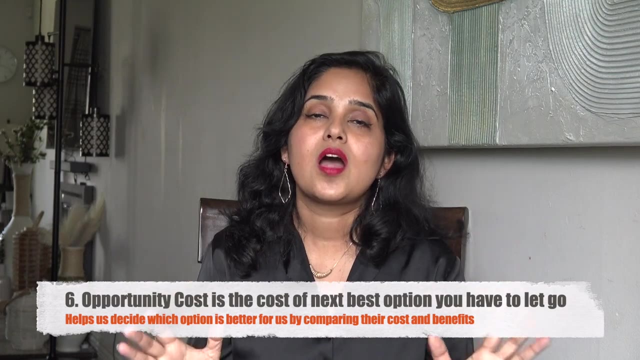 know about is called opportunity cost. Whenever you make a choice, you have to give up something else. The thing you give up is called the opportunity cost. So opportunity cost just refers to the cost of choosing one option over another and is a key economic concept. 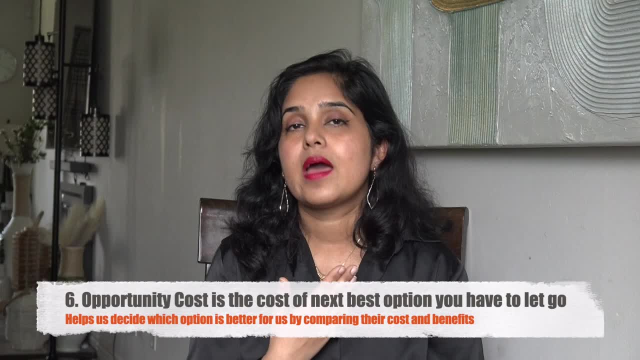 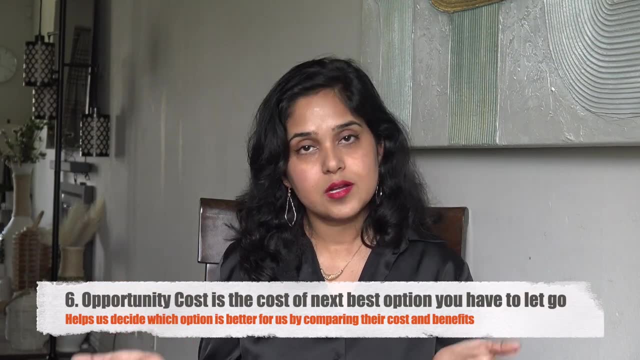 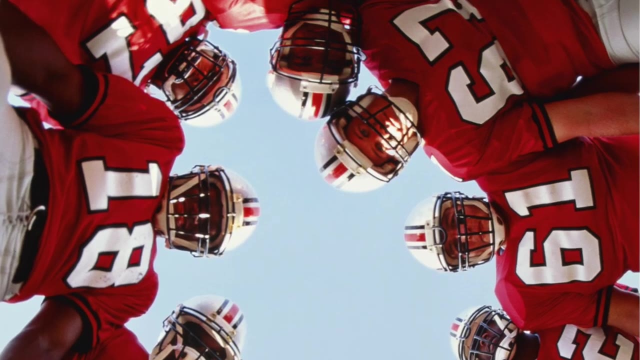 in decision making. When making decision, individual and businesses must weigh the potential benefits of each option against the opportunity cost of choosing the other option. A student deciding whether to attend a football game or to study for an upcoming exam. If he decides to attend the football game, the opportunity cost is the time and effort they 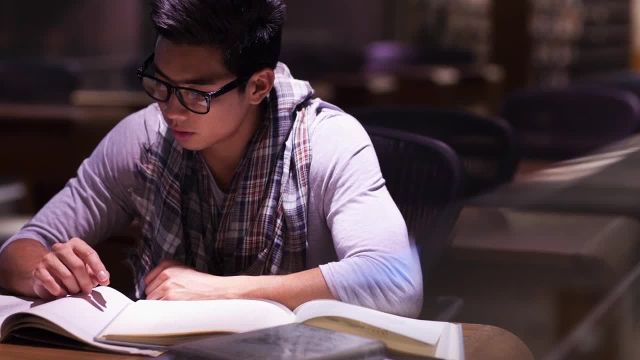 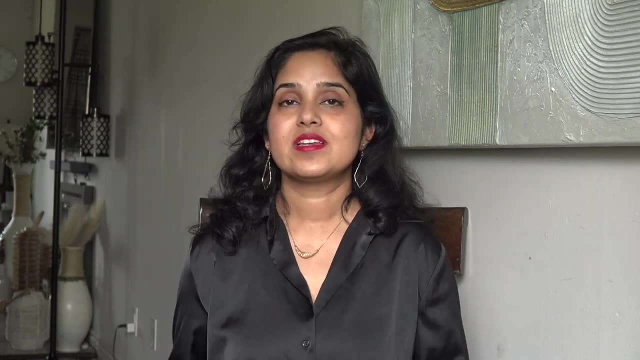 could have spent Studying for the exam. Alternatively, if the student decides to study for the exam, the opportunity cost is the experience of attending the football game and the social interaction that comes with it. So, in this case, the opportunity cost of attending the football. 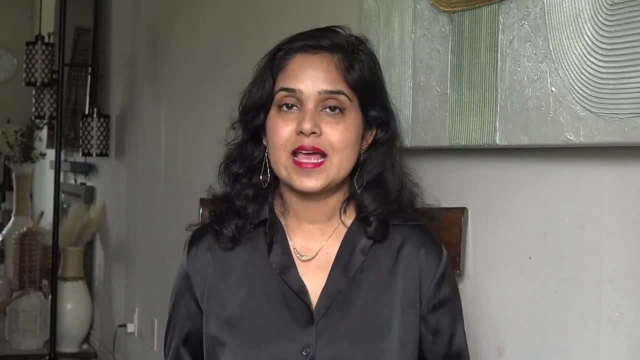 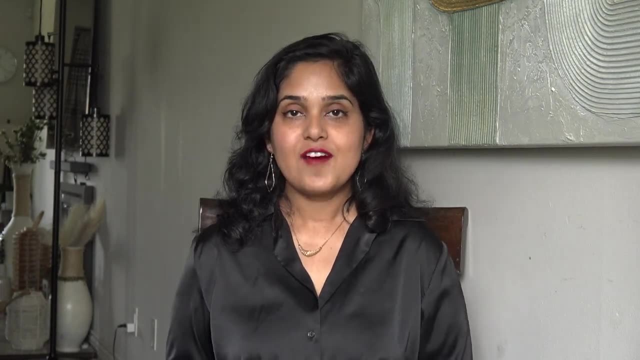 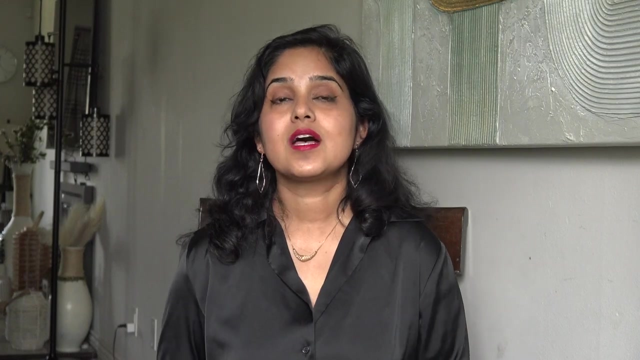 game is the lower grade that the student may receive on the exam. Similarly, the opportunity cost of studying for the exam is the fun and enjoyment the student would have had by attending a football game. So opportunity cost is important to consider because it helps us to make better decisions by weighing 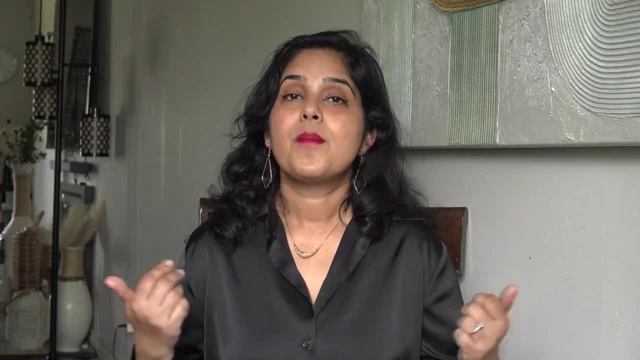 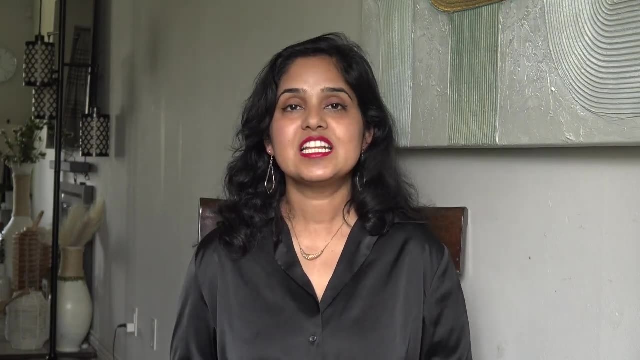 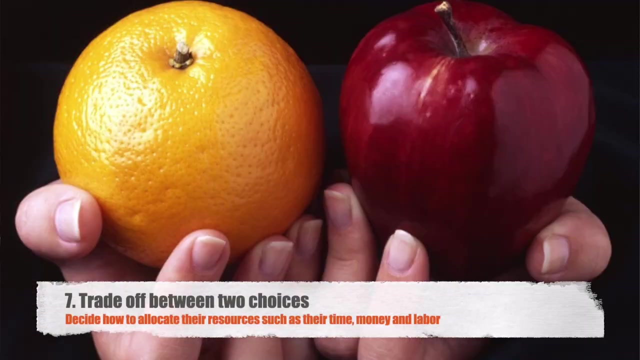 the potential benefits and cost of different options. By understanding this concept, we can make more informed decisions and ultimately achieve our goals more effectively. Another related concept is called trade-off. When you have to choose between two things, you have to give up one thing to get the other. This is called a trade-off. 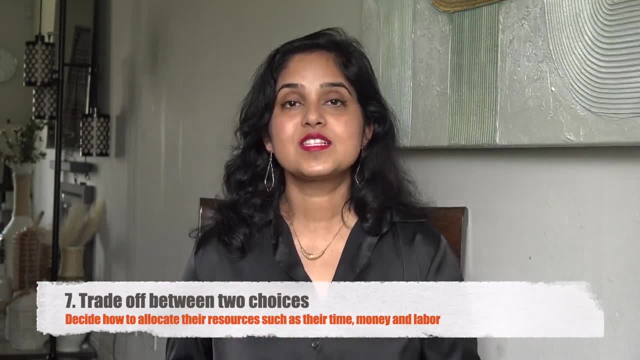 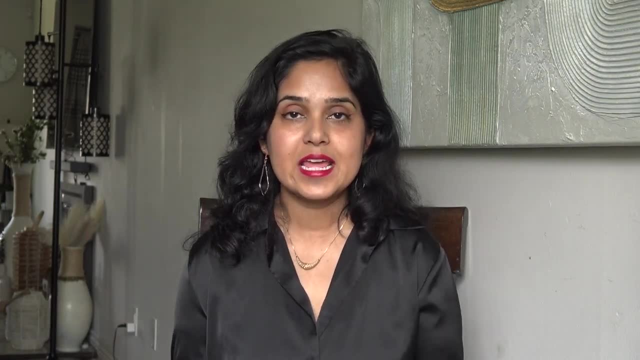 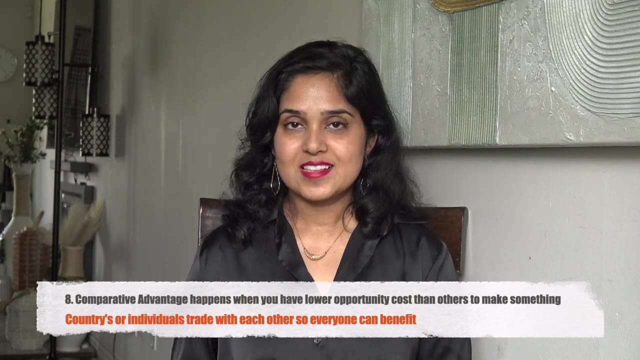 In economics, individuals and businesses must make trade-off when deciding how to allocate resources such as their time, money and labor. Lastly, we have something called comparative advantage. So how do I explain this in simple words? Hmm, Okay, so this is a difficult term. 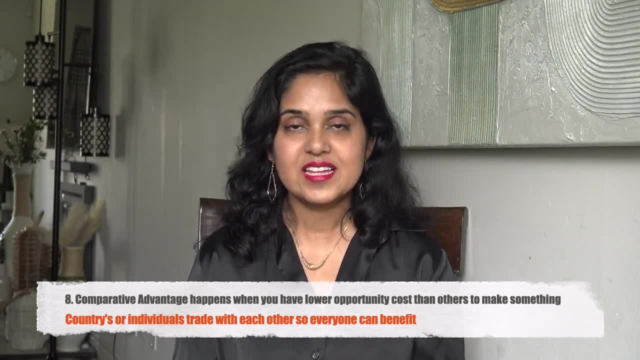 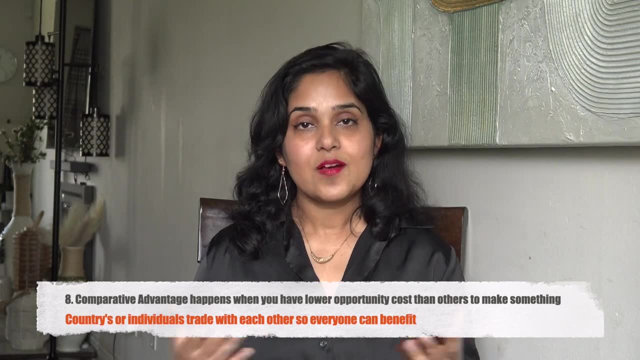 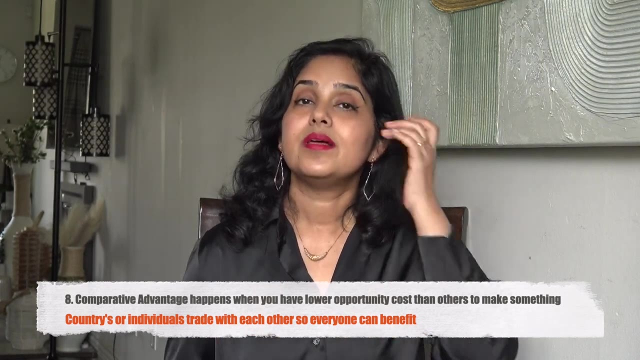 but it just tells you that everyone is better at doing something than others. Comparative advantage is when someone's better at making something than someone else. This is why countries trade with each other, So comparative advantage refers to the ability of a country or an individual to produce a. 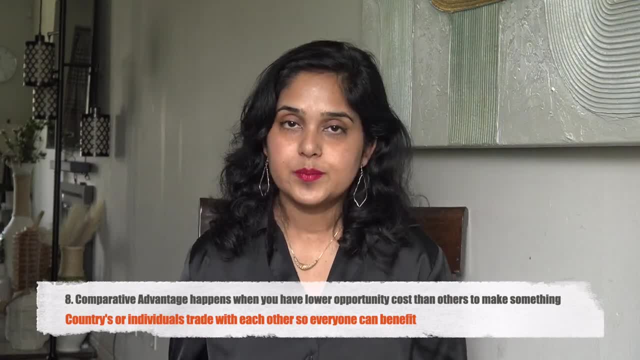 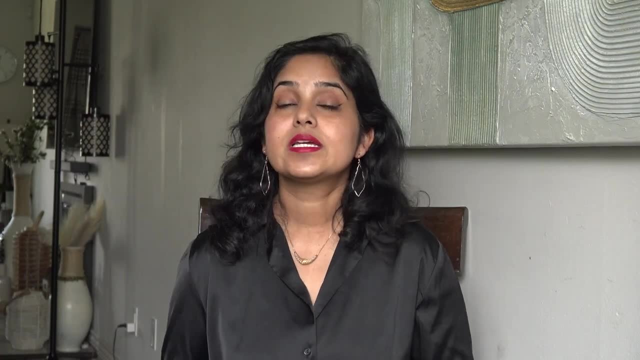 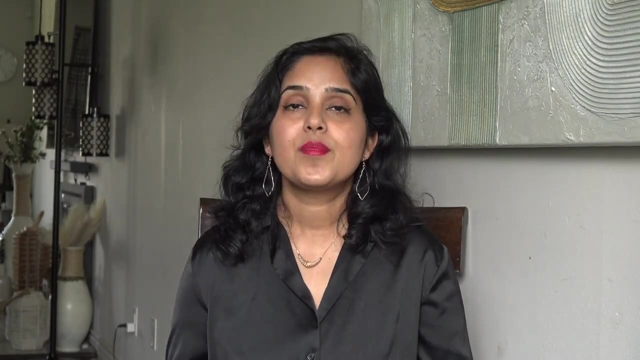 good or services at a lower opportunity cost than other person or country would, so that they can trade with each other and get mutual benefit. A person or a country can have absolute advantage in making all those things better and faster or more efficiently, but they have to choose which one they're best at. So how does this benefit the? 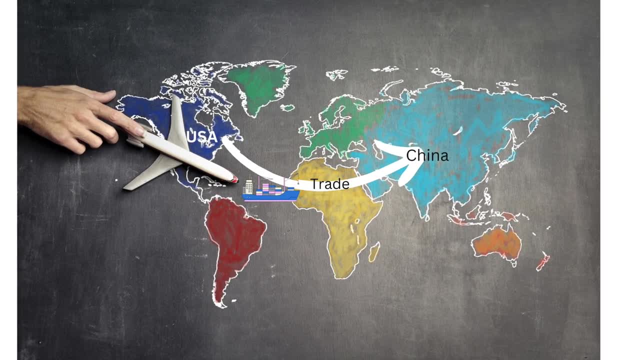 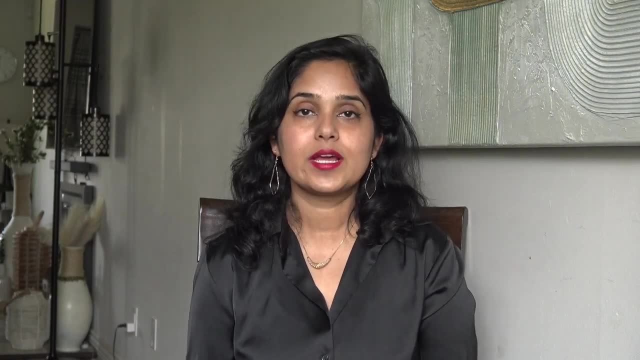 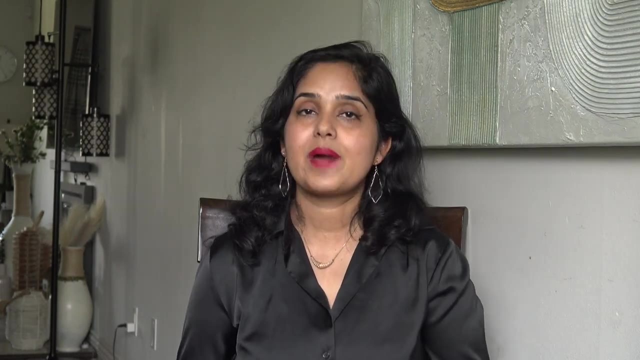 countries. Let's understand this with the help of China and US trade. So China and US have different comparative advantages in the global economy. China has a comparative advantage in producing low-cost manufactured goods, while the US has a comparative advantage in producing. 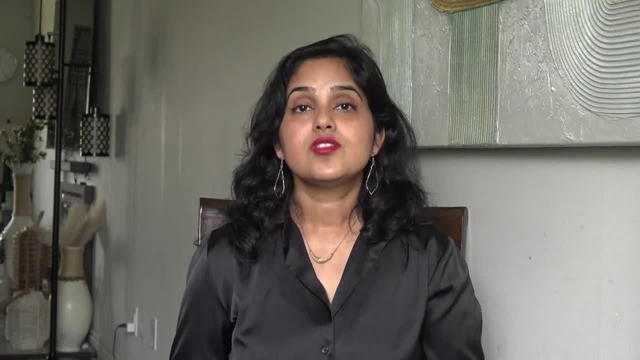 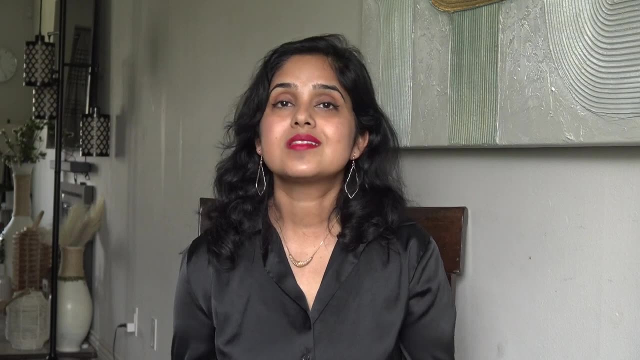 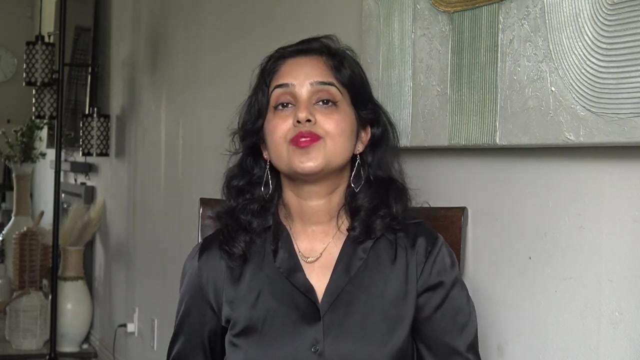 high-tech goods and services. So, for example, China produces a large amount of electronics and textiles, and it is able to produce these goods at a lower cost than many other countries due to its lower labor costs. The US, on the other hand, has a comparative advantage.